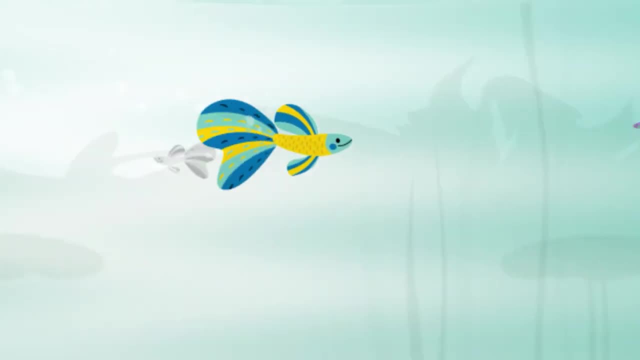 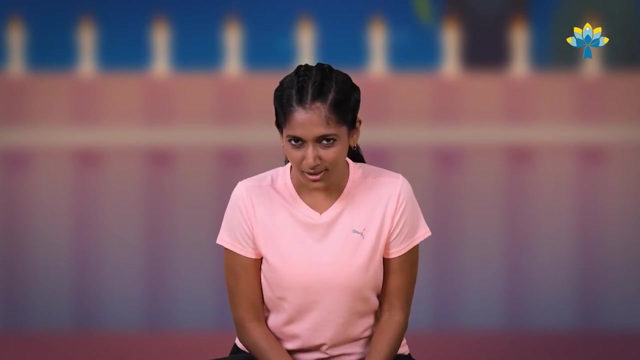 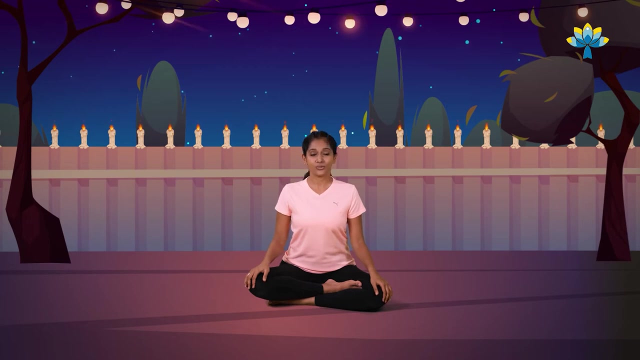 Namaste and welcome to Yoga Gappi. I am Rashmi. Are you ready to become strong and focused? Yoga Gappis? We are going to practice the candle breath so that you can become strong and focused. I want you to sit down on your mat with your back straight and your legs. 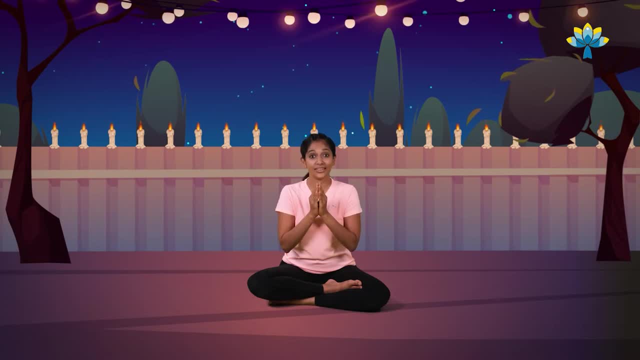 crossed and let's join your palms together. Now we are going to breathe in and make a long, big flame with your arms. Let's breathe in and you are going to hold your breath there and when I tell you to breathe out, you are going to bring your hands down and go, Are? 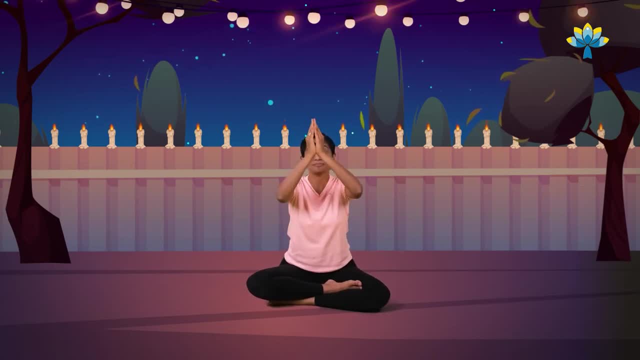 you ready to try it with me? Let's go. Let's breathe in and go. Very nice, Let's try that one more time, Breathe in and let's go One more time. Let's breathe in and breathe out. 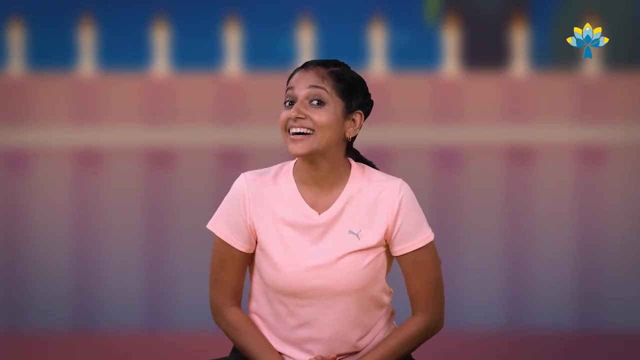 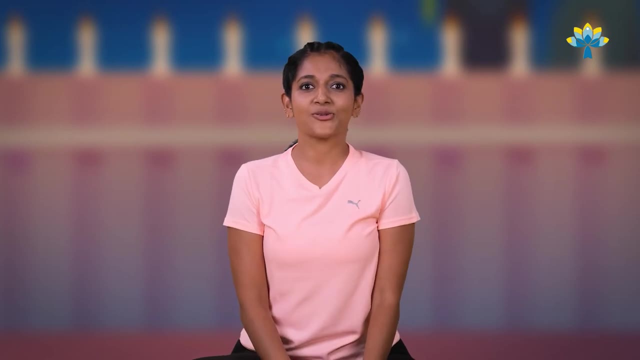 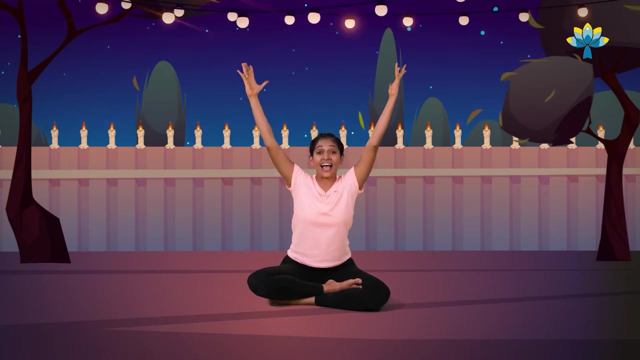 Now, when do you blow out candles On your birthdays? Yes, So we are going to practice the candle breath and we are going to sing the happy birthday song with it. Are you ready? Let's breathe in and sing happy birthday to you One more time. Breathe in and sing happy birthday to you. Breathe out. 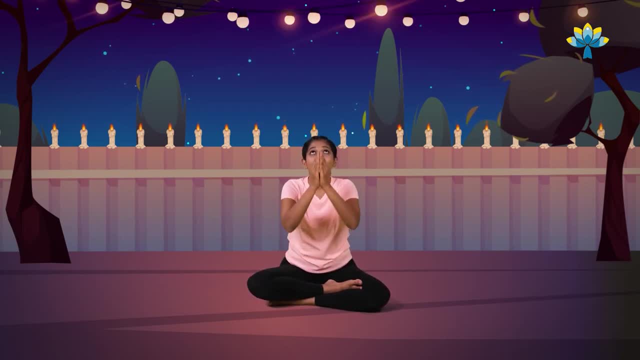 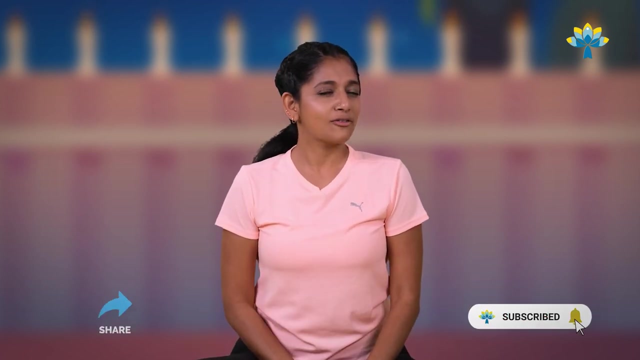 One more time, One last time. Breathe in and sing happy birthday to you. Breathe out Very good, I hope you enjoyed this breathing exercise and your lungs are feeling very, very strong. Remember to practice the candle breath before you have to blow out all your birthday candles or if